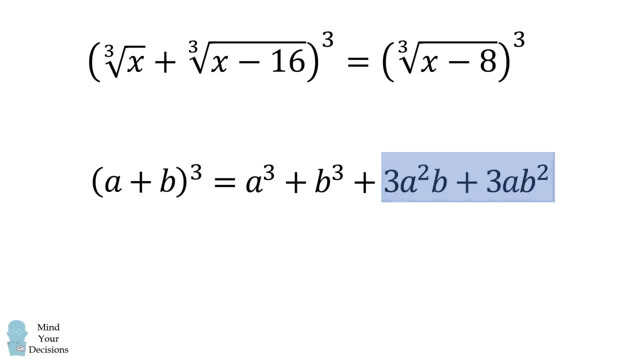 We will now factor the final two terms To do that. we'll write 3a squared b as 3a times a times b. We'll write 3ab squared as 3a times b times b. The first term has a factor of 3ab and the second term also has a factor of 3ab. 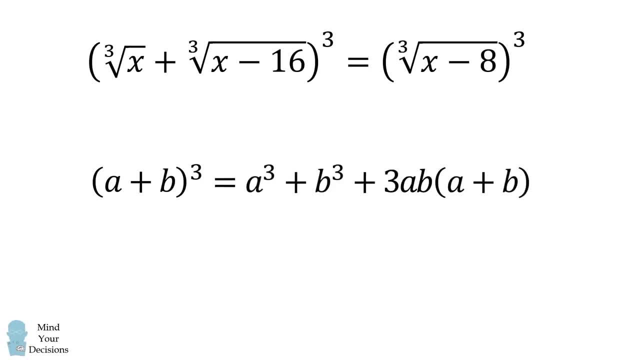 We've factored these out to get 3ab multiplied by a plus b. Now go back to the original equation. Let the cube root of x be equal to a. Let the cube root of x minus 16 be equal to b. From the original equation we know the sum of a and b is equal to the cube root of x minus 8.. 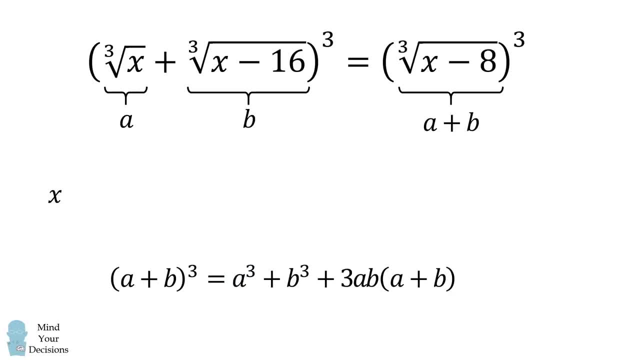 So a cubed is equal to x. We then add b cubed, Which is equal to x minus 16.. We then have 3 multiplied by a, multiplied by b. We write that out And then we have the sum of a and b. 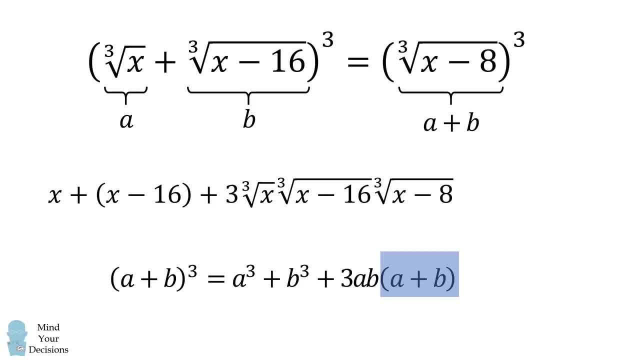 And we know that's equal to the cube root of x minus 8.. This is all equal to the cube root of x minus 8 being cubed, So this will be equal to exactly x minus 8.. Let's now simplify this equation. 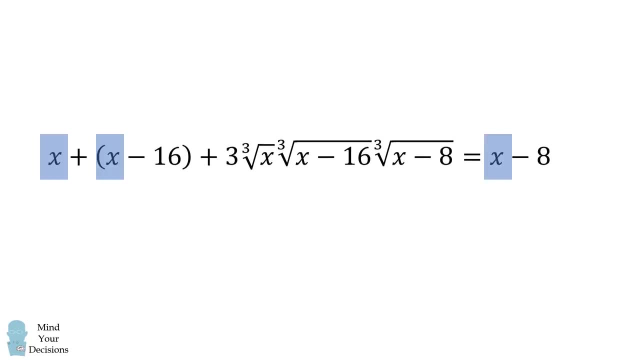 We have 2x on the left hand side and we have x on the right hand side. We'll subtract 2x from both sides of the equation, so the right hand side becomes negative x. We then have negative 16 on the left hand side and negative 8 on the right hand side. 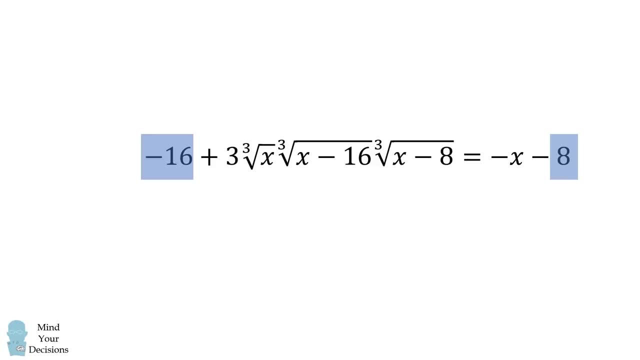 We will add 16 to both sides of this equation, so we have negative x plus 8.. From here, negative x plus 8 is equal to the opposite of x minus 8.. We will now cube both sides of this equation. The right hand side becomes the opposite of the quantity x minus 8 cubed. 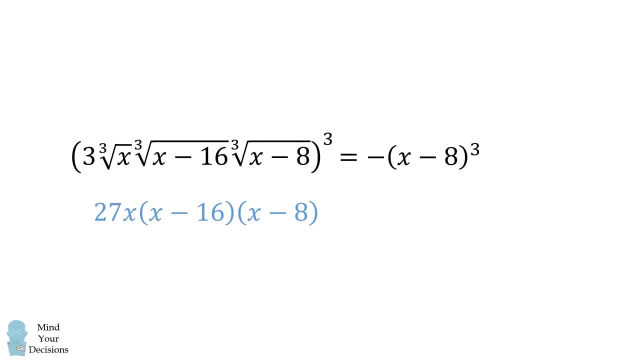 We then cube each term on the left hand side. We get 27x multiplied by the quantity x minus 16 multiplied by the quantity x minus 8.. From here we will add x minus 8, the quantity cubed to both sides of the equation. 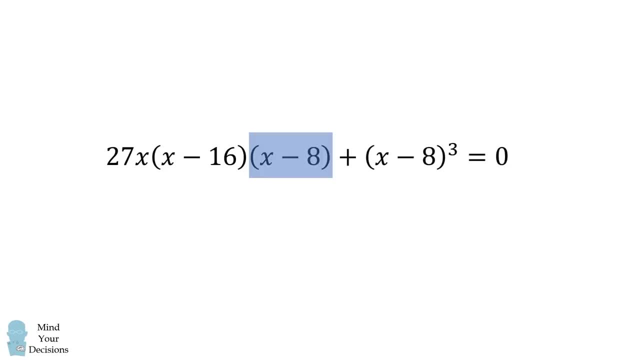 We will now add x minus 8, the quantity cubed to both sides of the equation. From here we will add x minus 8, the quantity cubed to both sides of the equation. From here we can factor a term of x minus 8.. 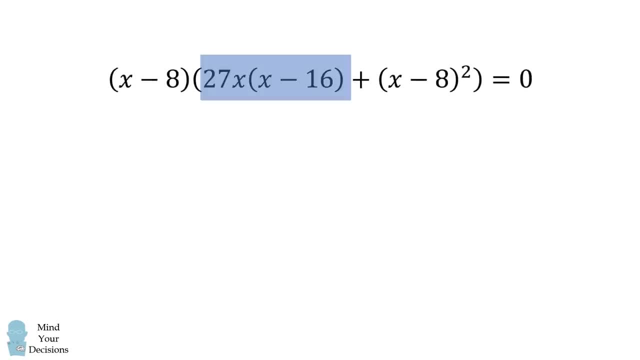 We now need to simplify the remaining terms. We'll expand out 27x multiplied by x minus 16.. Then we will expand out the binomial x minus 8 squared. From here we will group like terms. So we group the x squared terms, we group the x terms and then we have the constant term. 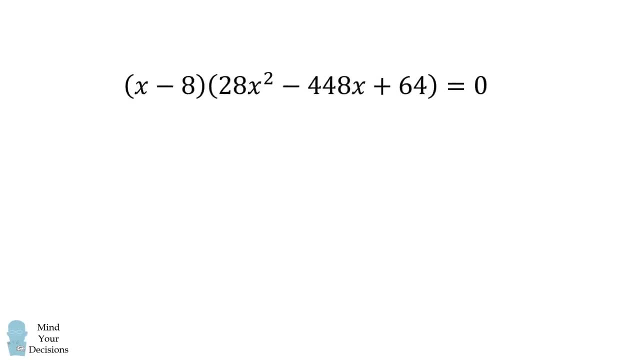 So we're making good progress. We can make one more simplification. Each of these terms has a factor of 4.. They're each divisible by 4. So we'll factor out the 4.. To solve this equation, we have two possibilities. 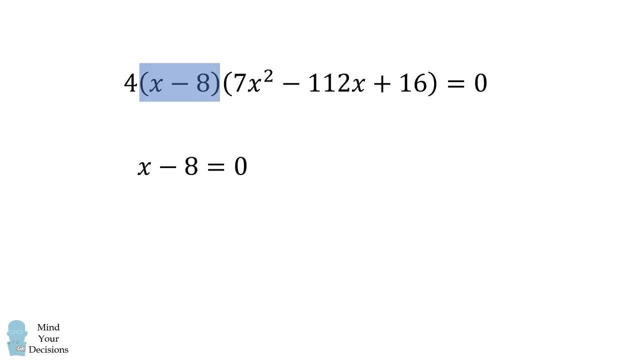 Either x minus 8 is equal to 0, in that case x is equal to 8, so that's one solution. or we have this: quadratic is equal to 0.. To solve this quadratic equation we'll use Brahmagupta's quadratic formula. 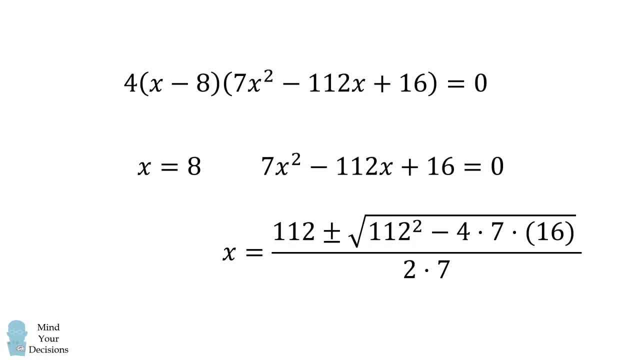 We'll substitute in. Now we just need to carefully simplify this equation. It's a matter of arithmetic. We'll just carefully simplify and we'll get that x is equal to 8.. Then we find out that x is equal to 1 over 8, plus or minus 12 over 7, multiplied by the square root of 21,. 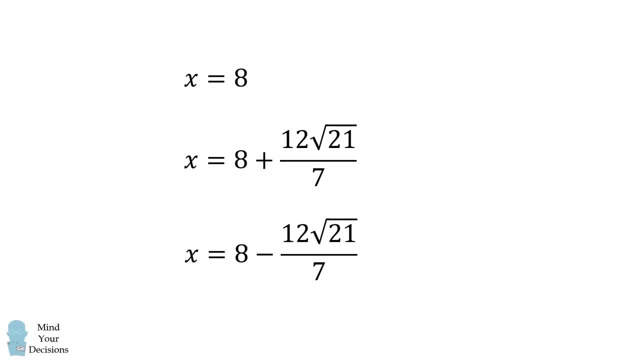 plus x into 1. overека plus-�� are equal to 1 over a square root of 21, or plus or minus 12 over seven multiplied by the square root of 21.. So there are three solutions to the original equation. x is equal to 8,. 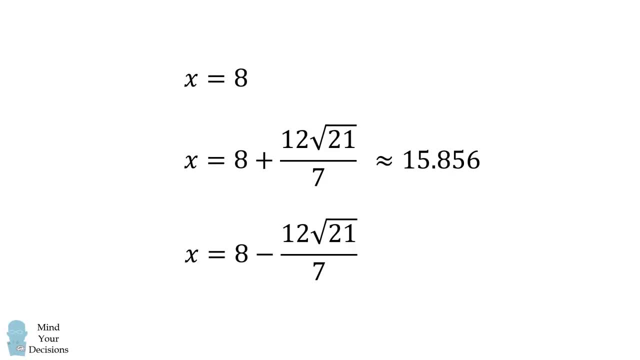 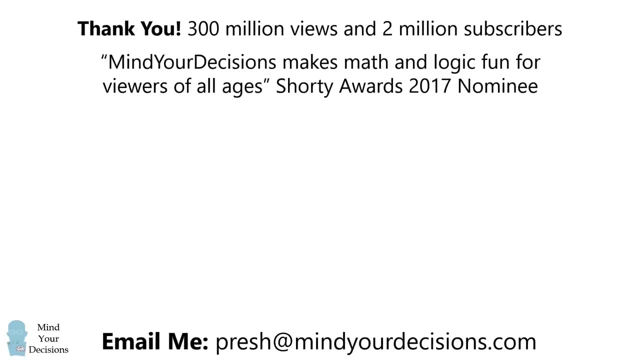 x is equal to 8 plus 12 over 7 multiplied by the square root of 21,, which is approximately equal to 15.856, and And that's the answer. Thanks for making us one of the best communities on YouTube. See you next. episode of Mind Your Decisions, where we solve the world's problems. one video. at a time.